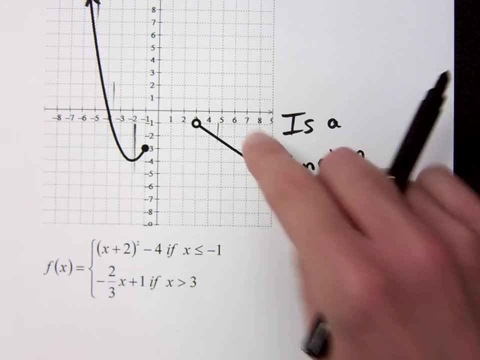 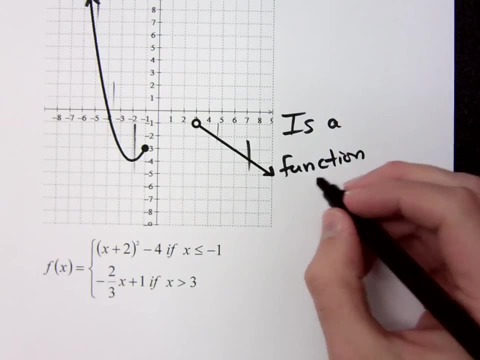 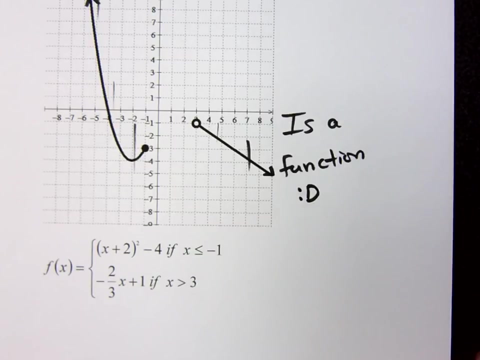 not at these end points that I have. This guy's going to keep going over Over here. No, This is going to keep going up and up. Now let's talk about the domain. The domain can be kind of weird, so let's talk about this guy. The domain is the set. 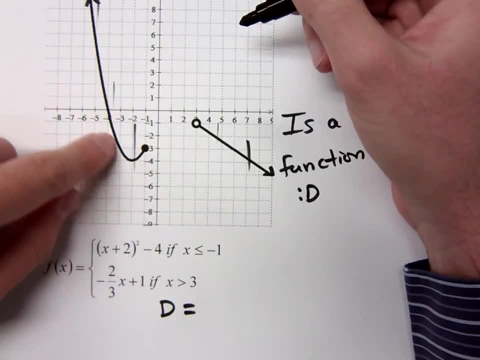 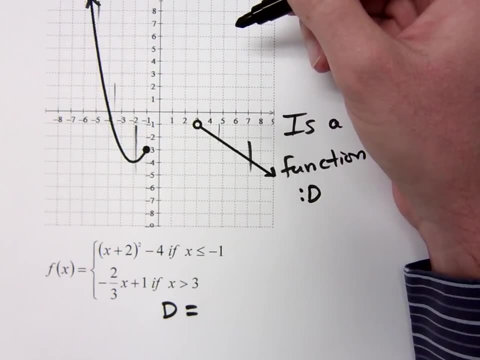 of x's right. So this guy, what you need to understand is he's going up and up and up and he's getting further and further out to the left. It may be difficult to see that because of the steepness, but he is going up and up and up and he's getting further. 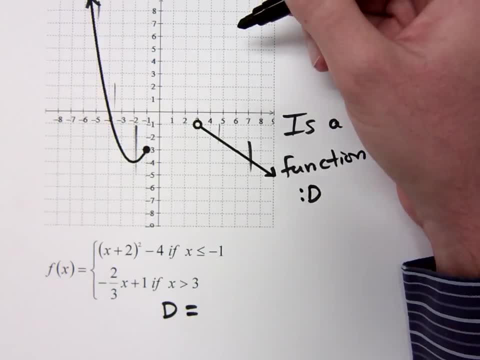 and further out to the left. It may be difficult to see that because of the steepness, but he is going up and up and up and he's getting further and further out to the left. So when I put this on the x-axis, if I were to smash all this onto the x-axis- okay, this guy goes. 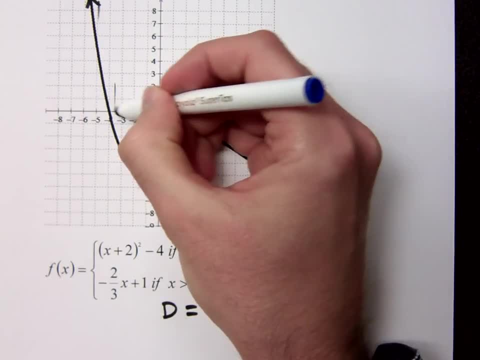 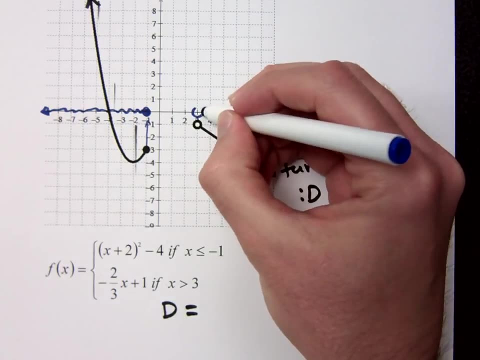 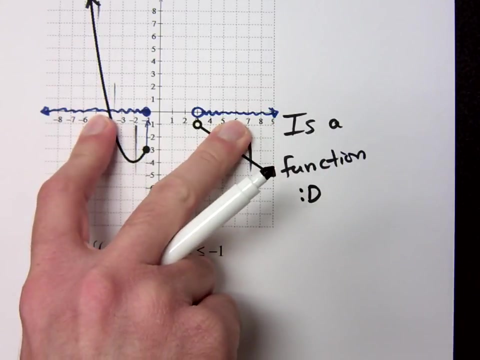 up here as a closed circle, and, you see, all these other points would be mapped out here, going all the way to the left, right Here, though I have an open circle here at three and I'm going all the way out to the right. How would you take this, this part of my domain? 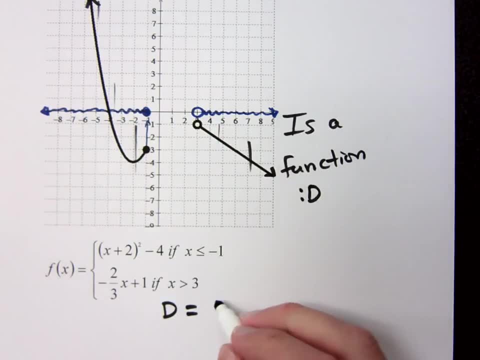 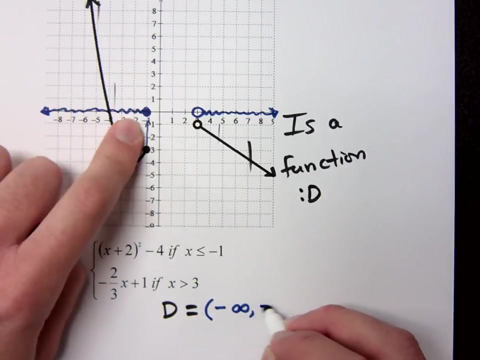 and write that using interval notation. Okay, Right, so what's on the left part, Parentheses? negative, infinity to no. I stop at negative one because I'm looking at the x values. I'm talking about the domain And you see I'm. 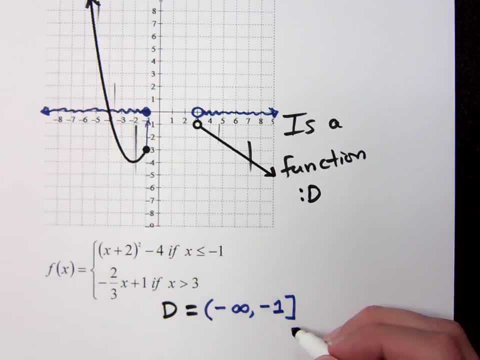 going from negative infinity to negative one. I pick back up where U Right, Okay, Okay. So I'm going to use parentheses. what Negative, Not negative Three? The x value is three going to infinity, Okay. 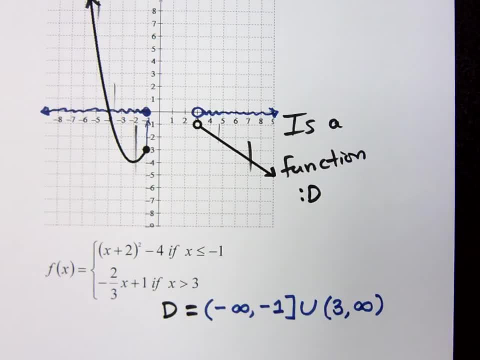 So why would you use one and not four? I'm looking at the x values Where it crossed. at four, I don't care where it crosses, I care about the x values that are used to make up this picture. Oh, I feel you because, oh, negative, one and three. that's the point, right there, That's.